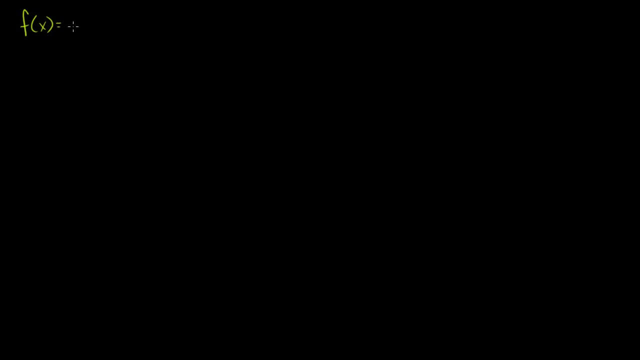 Let's say we've got the function f of x is equal to the natural log of x to the fourth plus 27.. And what we want to do is take its first and second derivatives and use as much of our techniques as we have at our disposal to attempt to graph it without a graphing. 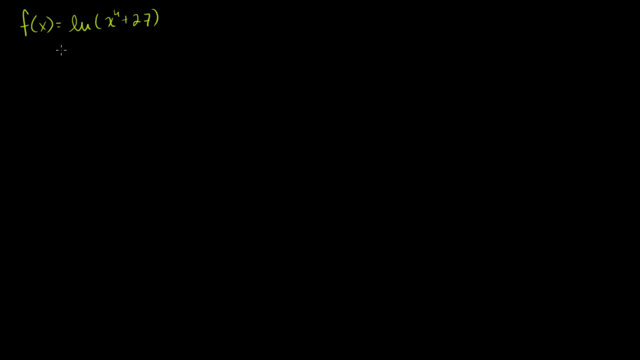 calculator. If we have time I'll take out the graphing calculator and see if our answer matches up. So a good place to start is to take the first derivative of this. Let me do that over here. So the derivative of f. well, you take the. 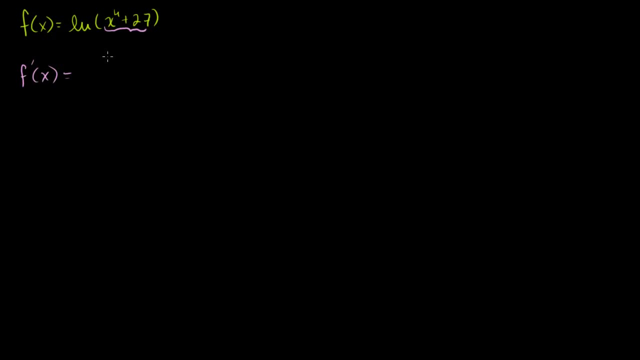 derivative of the inside. So take the derivative of that right there which is 4x to the third, and then multiply. it times the derivative of the outside with respect to the inside. So the derivative of natural log of x is 1 over x. 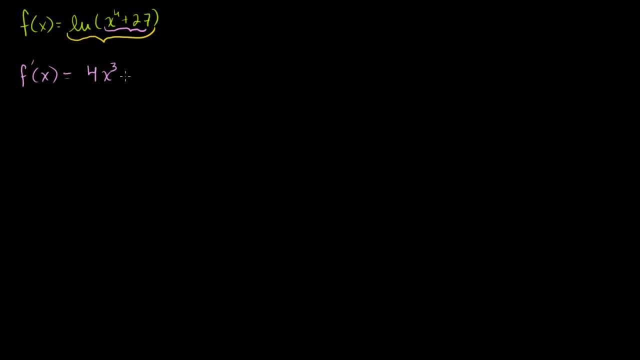 So the derivative of this whole thing with respect to this inside expression is going to be times 1 over x to the fourth plus 27.. If you found that confusing, you might want to re-watch the chain rule videos, But that's the first derivative of our function. 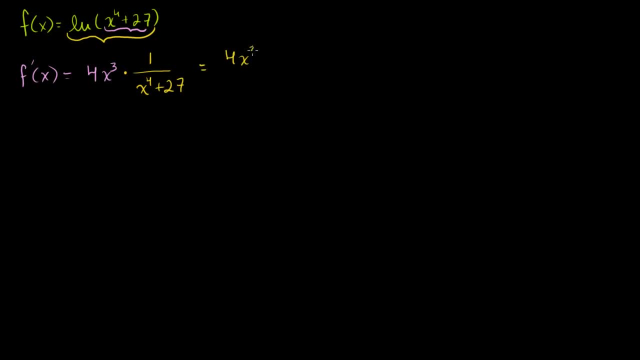 And I could rewrite this. This is equal to 4x to the third over x to the fourth plus 27.. Or I could write it as 4x to the third times x to the fourth plus 27 to the negative 1.. 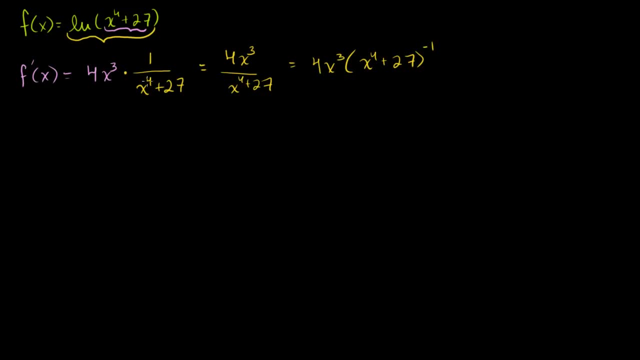 All three of these expressions are equivalent. I'm just writing, I've multiplied it out, Or I could write this as a negative exponent, or I could write this as a fraction, with this in the denominator. They're all equivalent. So that's our first derivative. 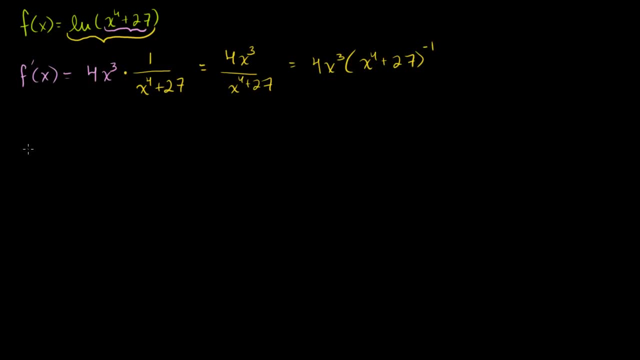 Let's do our second derivative, Our second derivative. this looks like it'll get a little bit hairier, So our second derivative is the derivative of this, So it's equal to. we can now use the product rule. it's the derivative of this first expression times the second. 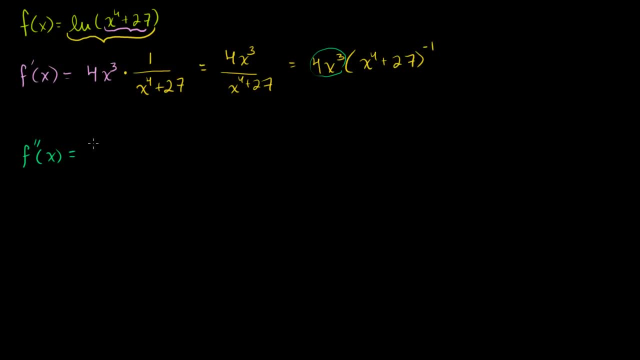 expression. So the derivative of this first expression, 3 times 4, is 12x squared right. We just decrement the 3 by 1.. Times the second expression: times x to the fourth, plus 27 to the minus 1.. 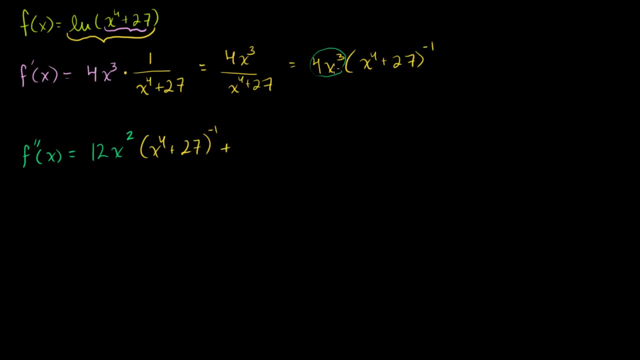 And then to that we want to add just the first expression, not its derivative. so just 4x to the third times, the derivative of the second expression And the derivative of the second expression. we could take the derivative of the inside, which is just 4x to. 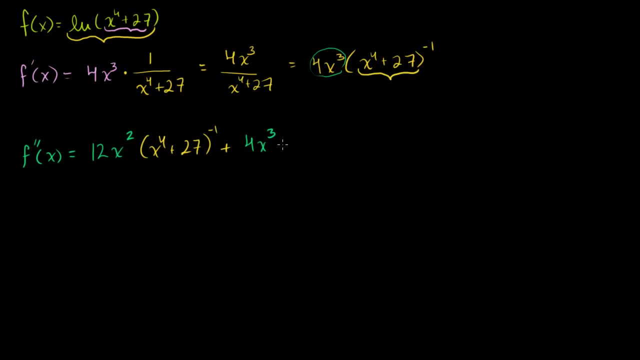 the third. This derivative of 27 is just 0. So it's times 4x to the third, times the derivative of this whole thing with respect to the inside So times. so you take this exponent, put it out front. 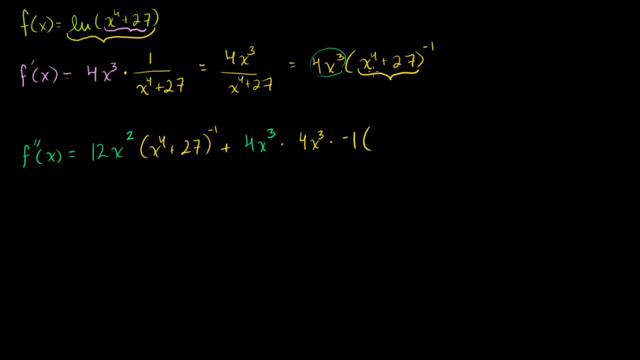 So times minus 1, times this whole thing, x to the fourth, plus 27, to the. we decrement this by one more, so minus 2.. So let's see if I can simplify this expression a little bit. So this is equal to. 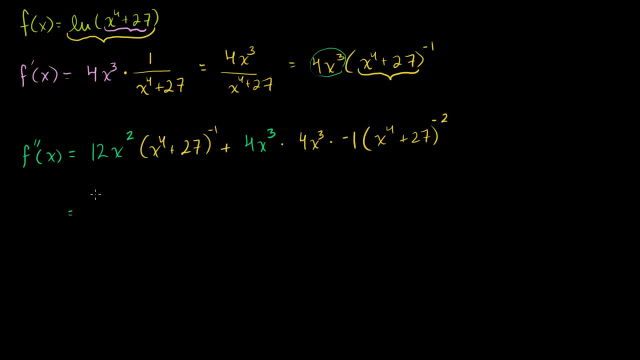 So this right here is equal to, Equal to 12x squared over this thing, x to the fourth plus 27.. And then let's see we're going to have a minus here. So it's minus. you multiply these two guys. 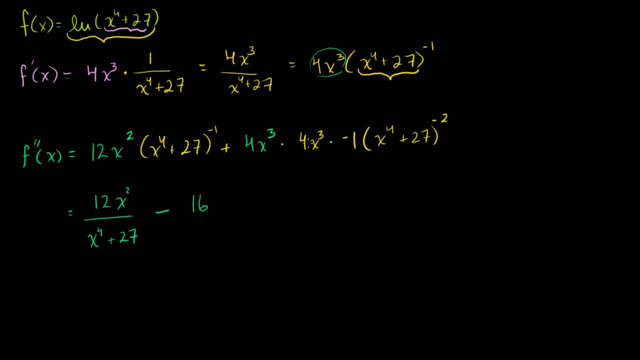 4 times 4 is 16.. 16x to the third times x to the third is x to the sixth. over this thing squared over x to the fourth plus 27 squared. That's just an another way to rewrite that expression. right there, right. 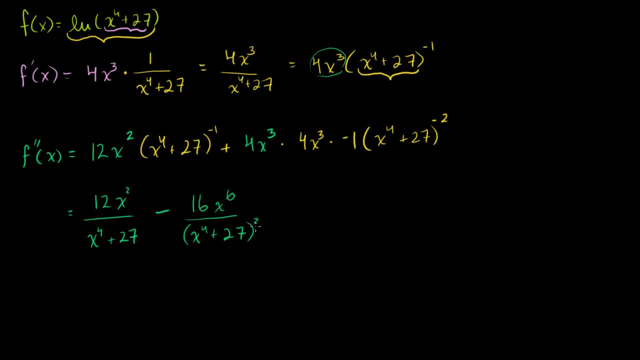 To the minus 2, you could just put it in the denominator and make it to a positive 2 in the denominator. Same thing. Now, if you've seen these problems in the past, we always want to set these things equal to 0.. 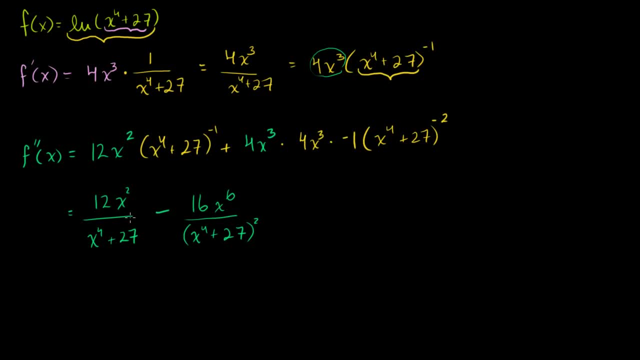 We want to solve for x equals 0.. So it'll be useful to have this expressed as just one fraction instead of the difference or the sum of two fractions. So what we could do is we could have a common denominator, So we could multiply both the numerator and denominator of. 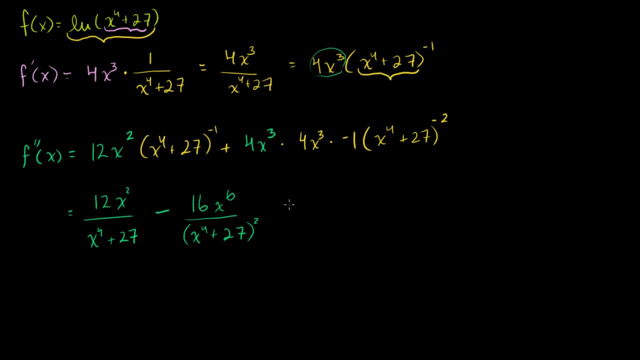 this expression by x to the fourth plus 27.. And what would we do? We could multiply both the numerator and denominator of this expression by x to the fourth plus 27.. So this is equal to: so if we multiply this first expression times x to the fourth plus 27,. 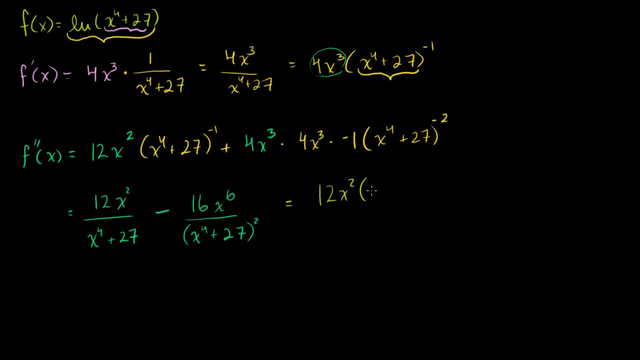 we get 12x squared times x to the fourth plus 27.. And then in the denominator you have x to the fourth plus 27 squared. All I did, I multiplied this numerator and this denominator by x to the fourth plus 27.. 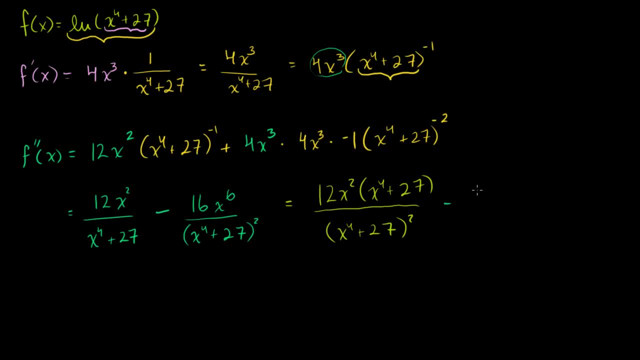 I didn't change it. And then we have that second term Minus 16x to the sixth, over x to the sixth. So that's 12x squared times x to the fourth, plus 27 squared. The whole reason why I did that. now I have a common denominator. 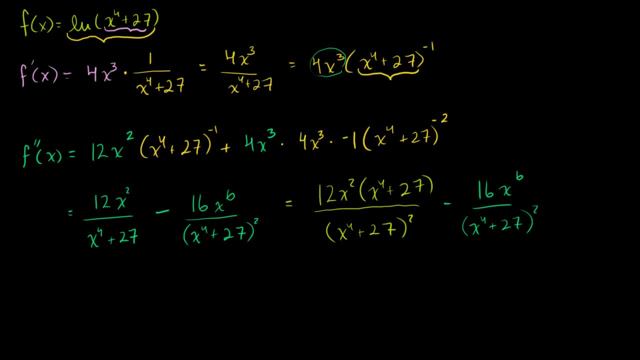 Now I can just add the numerators. So this is going to be equal to. let's see, let's multiply the denominator. We know what the denominator is. It is x to the fourth plus 27 squared. That's our denominator. 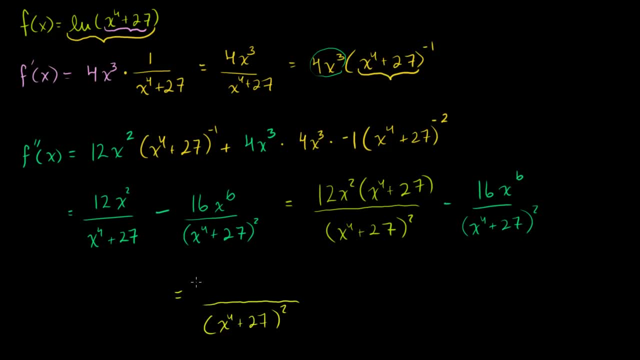 And then we can multiply this out. This is 12x squared times x to the fourth, So that's 12x to the sixth, plus 27 squared, So 27 times 12.. I don't even feel like multiplying 27 times 12,, so I'll just write that out. 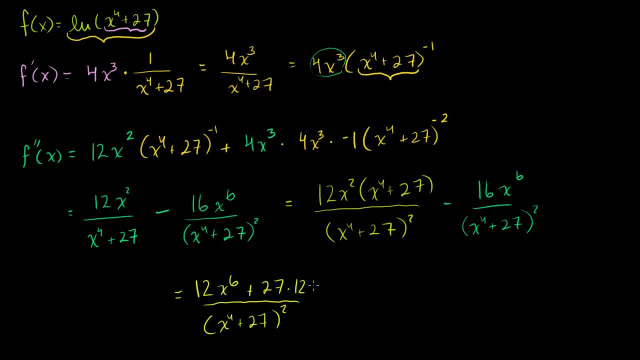 So plus 27 times 12x squared, I just multiply the 12x squared times this 27.. And then minus 16x to the sixth, Minus 16x to the sixth, And this simplifies too. Let's see if I can simplify this even further. 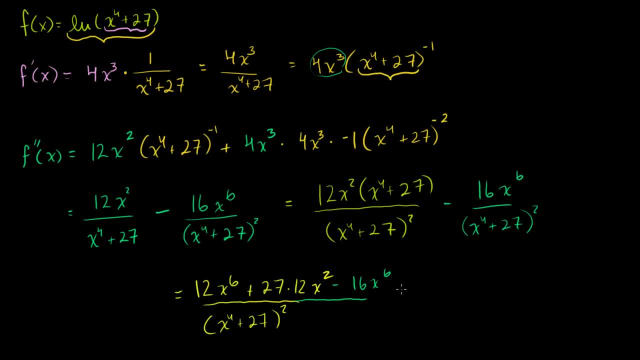 So I have an x to the sixth here, x to the sixth here. So this is equal to- I'll do this in pink. This is equal to the 27 times 12x squared. I don't feel like figuring that out right now. 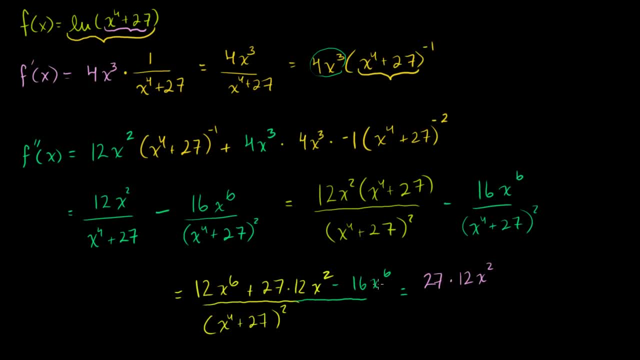 Times 12x squared, And then you have minus 16x to the sixth and plus 12x to the sixth. So you add those two, you get minus 4.. 12 minus 16 is minus 4.. x to the sixth. 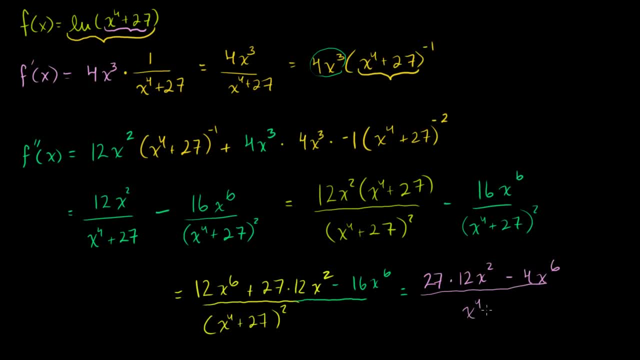 All of that over x to the fourth, plus 27 squared, And that is our second derivative. Now we've done all of the derivatives and this was actually a pretty hairy problem, And now we can solve for when the first and the second derivative is equal to 0.. 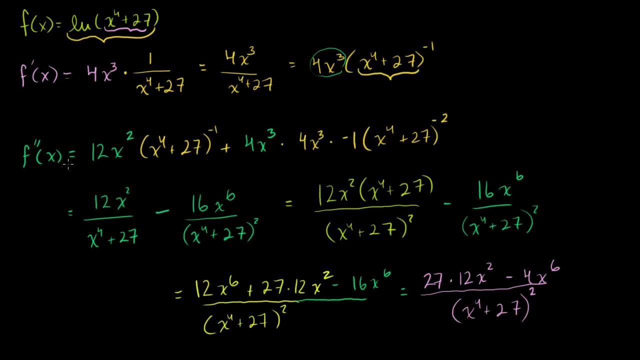 And we'll have our candidate. well, we'll know our critical points And then we'll have our candidate inflection points and see if we can make any headway from there. So first let's see where our first derivative is equal to 0 and get our critical points. 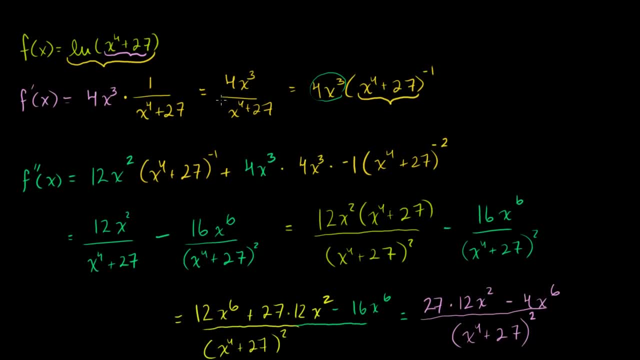 Or at least maybe also maybe where it's undefined. So this is equal to 0. If we want to set The only place that this can equal to 0 is if this numerator is equal to 0. This denominator- actually, if we are assuming we're dealing with real numbers, this term right here- is always going to be greater than or equal to 0 for any value of x, because it's an even exponent. 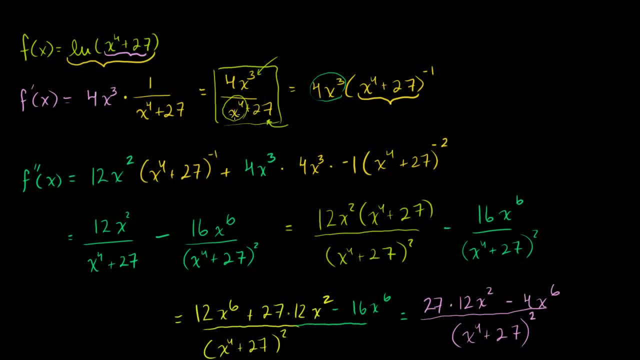 So this thing can never equal 0, right? Because you're adding 27 to something that's non-negative, So this will never equal 0. So this will also never be undefined. So there's no undefined critical points here, But we could set the numerator equal. 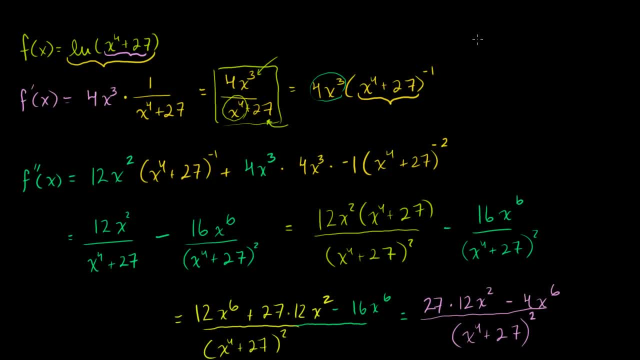 To 0 pretty easily. If we wanted to set this equal to 0, we just say 4x to the third is equal to 0. And we know what x value will make that equal to 0.. x has to be equal to 0. 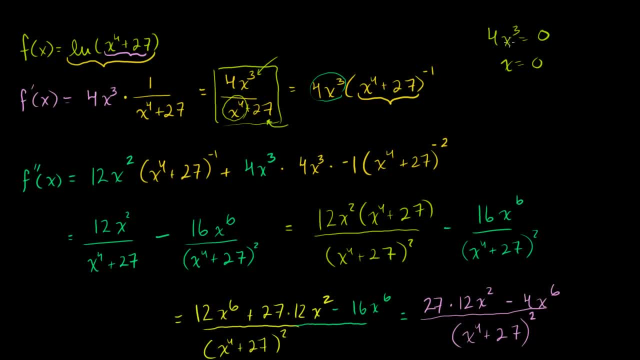 4 times something to the third is equal to 0.. That something has to be 0.. x to the third has to be 0.. x has to be 0.. So we can write: f, prime of 0 is equal to 0.. 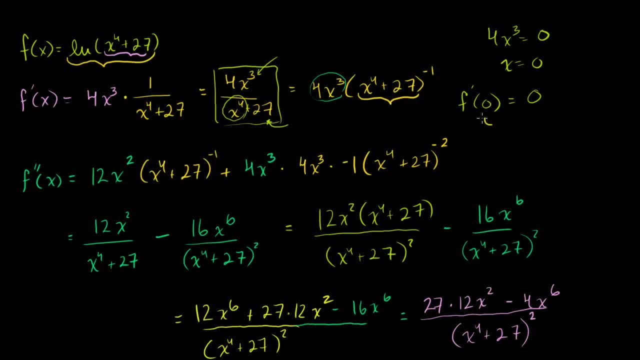 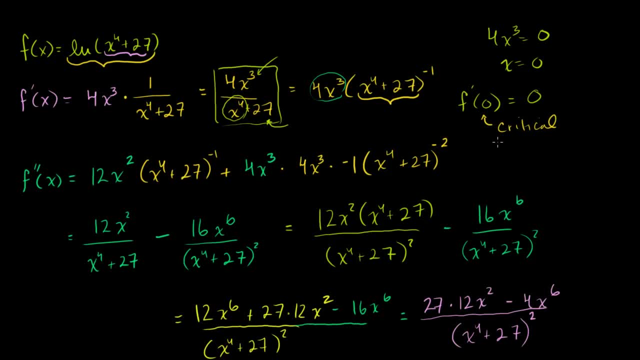 Or I mean, it could be, you know well, we'll explore it a little bit more. And actually, just so we get the coordinate, what's the coordinate? The coordinate x is 0.. And then y is the natural log. 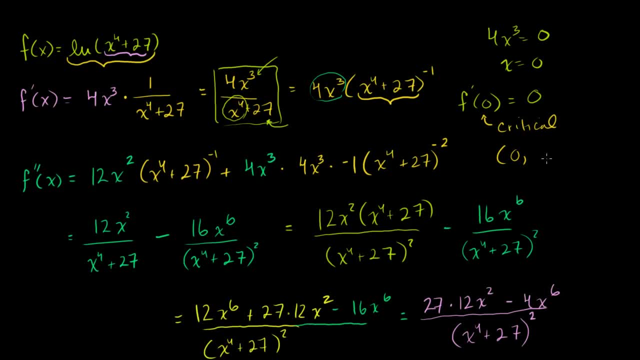 If x is 0, this just turns out. so it's the natural log of 27.. So it's the natural log of. let me figure out what that is and get the calculator out. I said I wouldn't use a graphing calculator, but I could use a regular calculator. 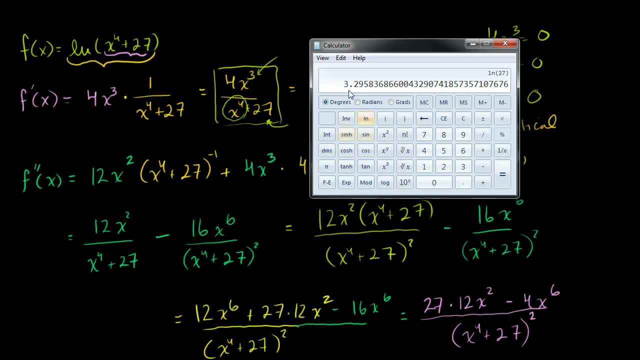 So 27.. If I were to take the natural log of that, it's like 3 point. well, for our purpose let's just call it 3.3.. We're just trying to get the general shape of the graph. 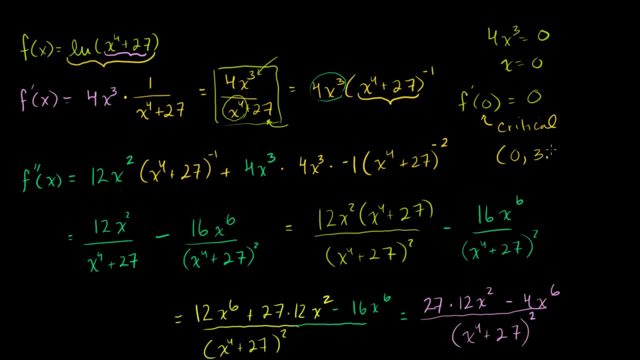 So 3.3.. 3 point- well, we could just say 29 and it could keep it kept going. So this is a critical point. right here The slope is 0. here Slope is equal to 0. at x is equal to 0.. 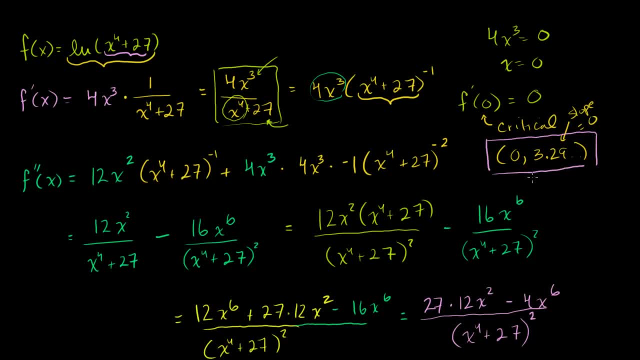 So this is one thing we want to block off And let's see if we can find any candidate inflection points. And remember, candidate inflection points are where the second derivative equals 0. Now, if the second derivative equals 0, that doesn't tell us that those are definitely. 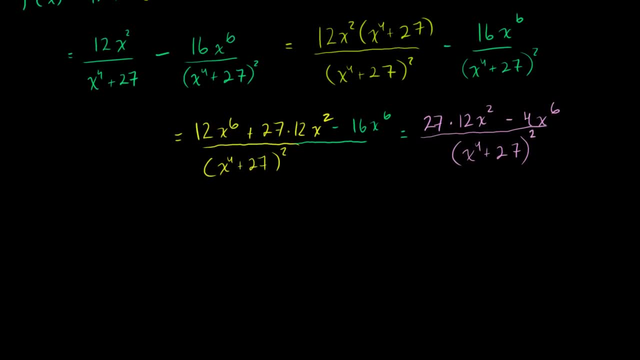 inflection points. Let me make this very clear. If let me write this, let me do it in a new color: If x is inflection inflection, then then the second derivative at x is going to be equal to 0.. 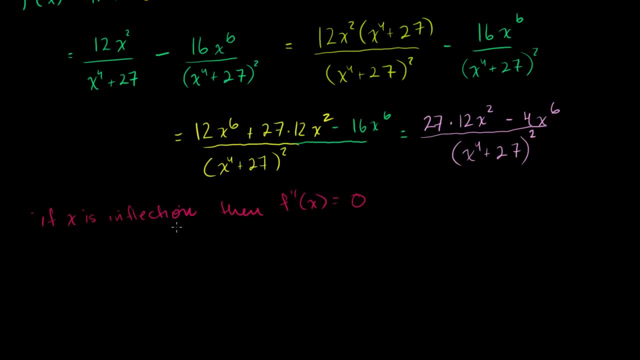 Because you're having a change. You're having a change in the concavity- I always say concavity but it's the concavity. You have a change in. the slope goes from either increasing to decreasing or from decreasing to increasing. But if the derivative is equal to 0, you cannot. the second derivative is equal to 0, you cannot. 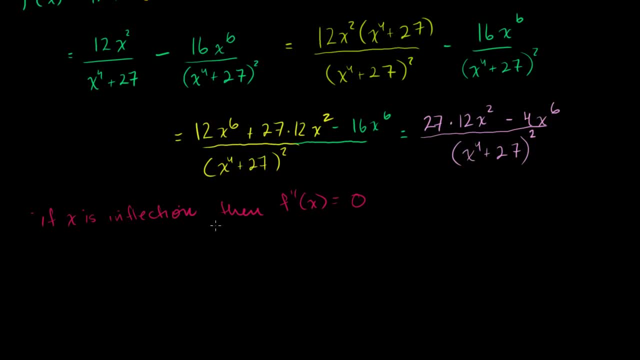 assume that it's an inflection point. So what we're going to do is we're going to find all of the points at which this is true, at which this is true, And then see if we actually do have a sign change in the second derivative at that point. 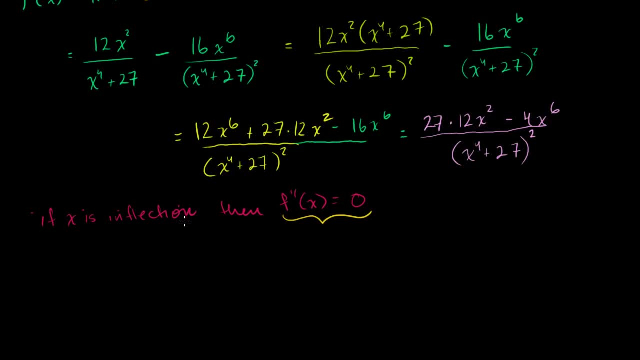 And only if you have a sign change, then you can say: it's true, Okay, It's an inflection point. So let's see if we can do that. So just because the second derivative is 0, that by itself does not tell you it's an inflection. 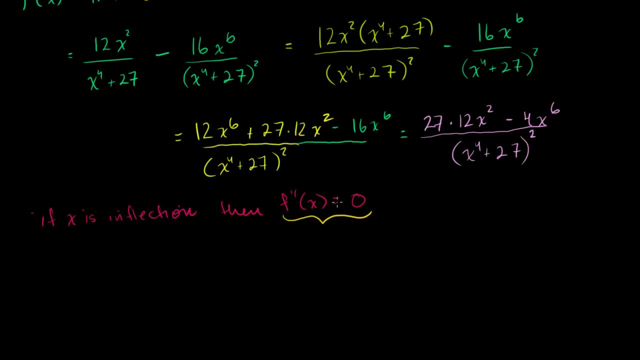 point. It has to have a second derivative of 0, and when you go above or below that x you have to. the second derivative has to actually change signs. Only then So we can say if f prime changes, changes signs around around x. 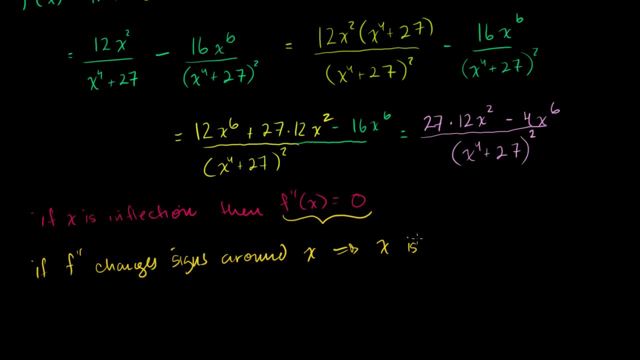 Then we can say that x is an inflection, X is inflection And if it's changing signs around x, then it's definitely going to be 0, right at x. But you have to actually see that if it's negative before x, it has to be positive after. 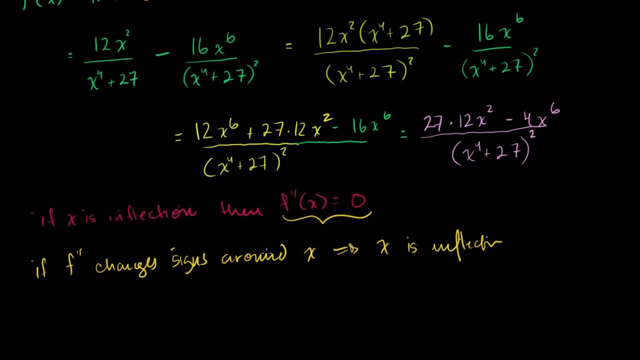 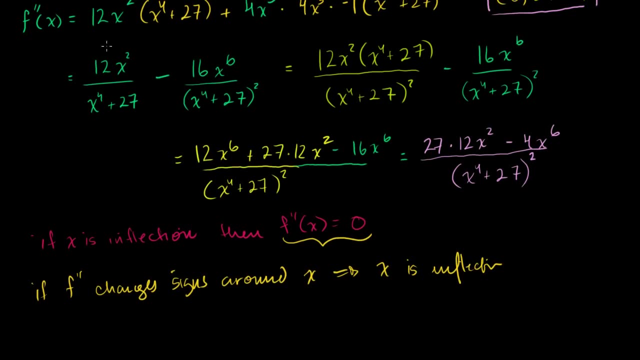 x, Or if it's positive before x, it has to be negative after x. Let's test that out. So the first thing we need to do is find these candidate points. Remember, the candidate points are where the second derivative is equal to 0.. 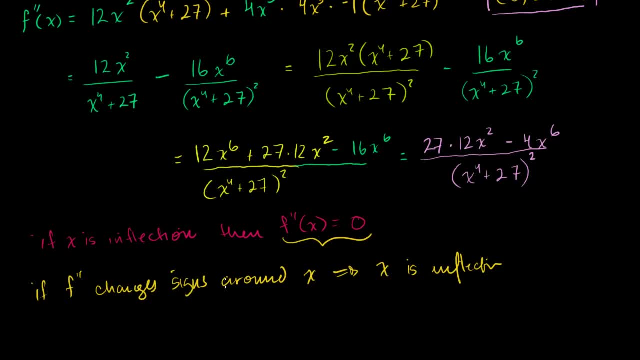 We're going to find those points and then see if this is true, That the sign actually changes. So we want to find where this thing over here is equal to 0. And once again, for this to be equal to 0, the numerator has to be equal to 0. 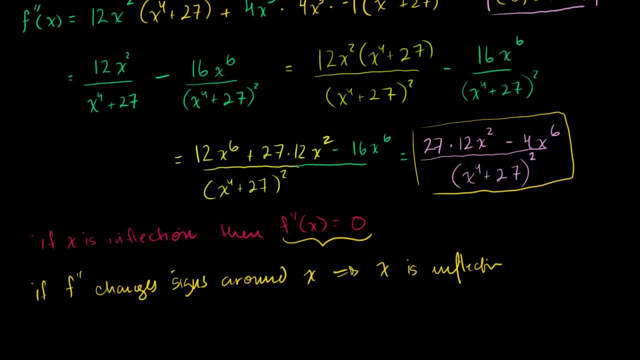 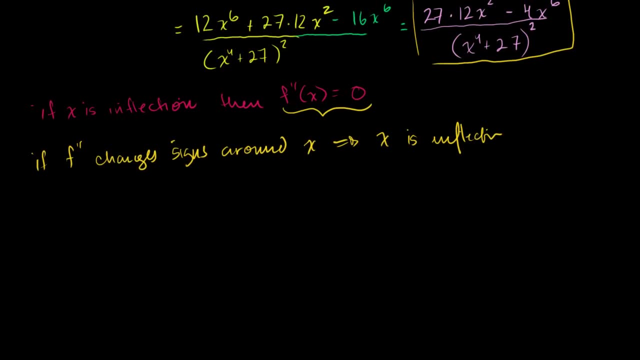 This denominator can never be equal to 0 if we're dealing with real numbers, which I think is a fair assumption. So let's see where our numerator can be equal to 0 for the second derivative. So let's set the second derivative, the numerator of the second derivative, 27 times 12x squared. 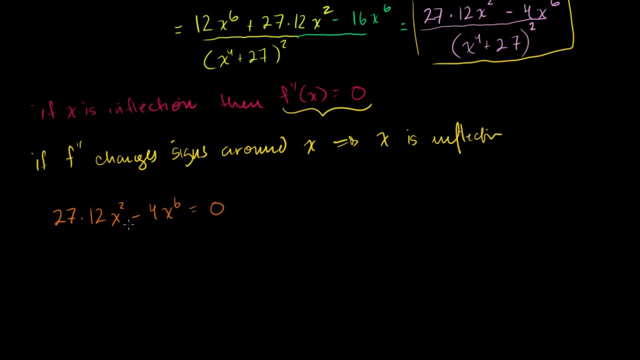 minus 4x to the sixth is equal to 0.. Okay, Remember, that's just the numerator of our second derivative. Any x that makes the numerator 0 is making the second derivative 0.. So let's factor out a 4x squared. 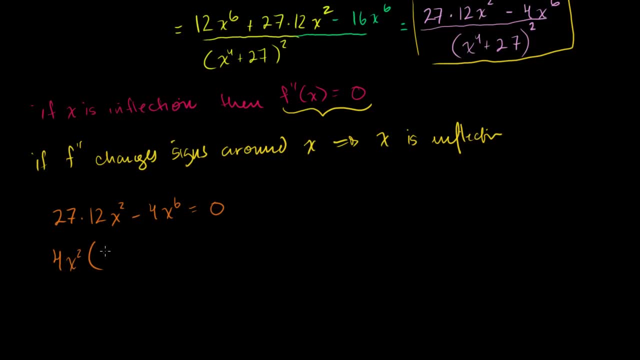 So 4x squared, Now we'll have 27 times. if we factor 4 out of the 12,, we'll just get a 3, and we factored out the x squared minus we factored out the 4,. we factored out an x squared, so we 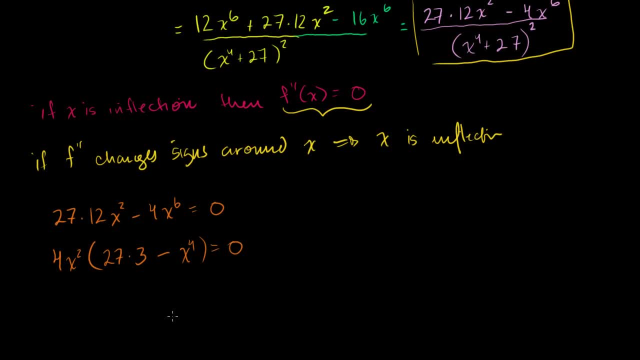 have x to the fourth is equal to 0. So the x's that will make this equal to 0 either will satisfy, either I'll switch colors. either 4x squared is equal to 0, or now 27 times 3, I can do that in my head, that's. 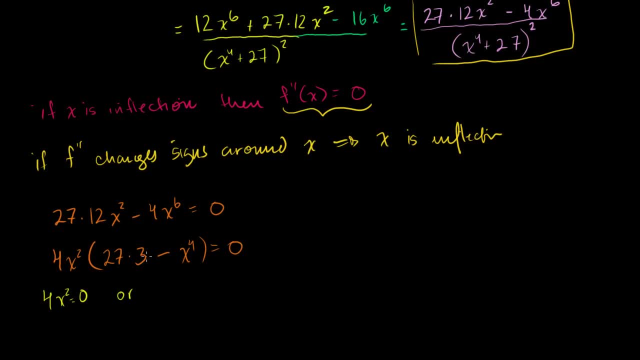 81.. 20 times 3 is 60,. 7 times 3 is 21,. 60 plus 21 is 81.. Or 81 minus x to the fourth is equal to 0.. Any x that satisfies either of these will make this entire expression equal to 0, because. 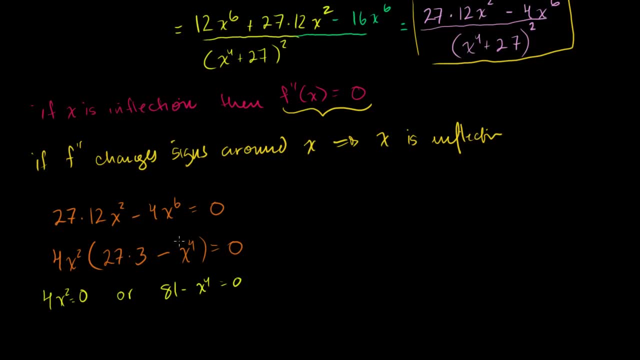 if this thing is 0, it's equal to 0.. Okay, Okay, If this thing is 0, the whole thing is going to be equal to 0.. If this thing is 0, the whole thing is going to be equal to 0.. 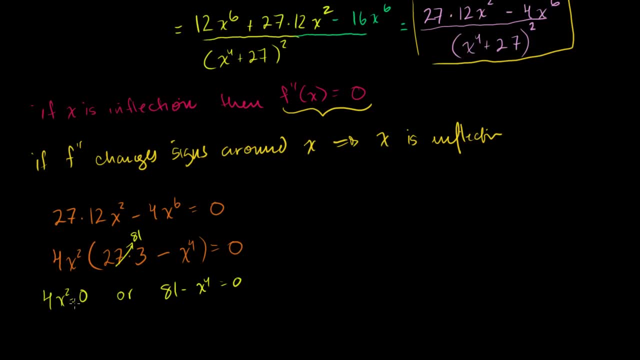 Let me be clear: this is 81 right there, So let's solve this. This is going to be 0 when x is equal when x is equal to 0 itself, This is going to be equal to 0 when x. let's see if we add x to the fourth, to both sides. 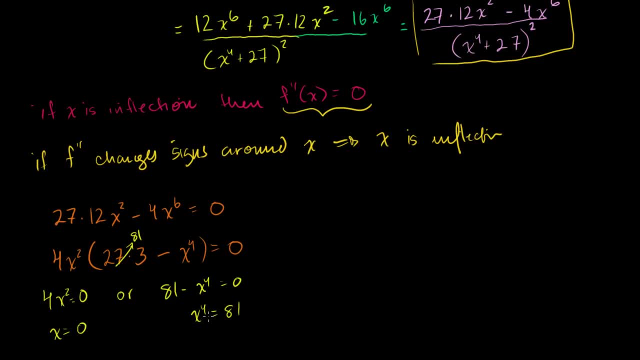 you get x to the fourth is equal to 81.. If we take the square root of both sides of this, you get x. squared is equal to 9, or so you get x is plus or minus 3.. x is equal to 9.. 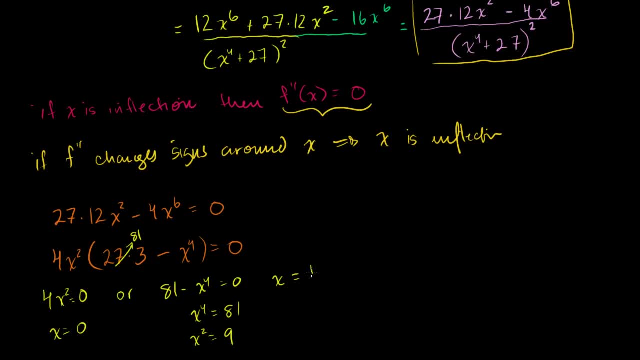 x is equal to plus or minus 3.. So these are our candidate inflection points: x is equal to 0,. x is equal to plus 3, or x is equal to minus 3.. So what we have to do now is to see whether the second derivative changes signs around. 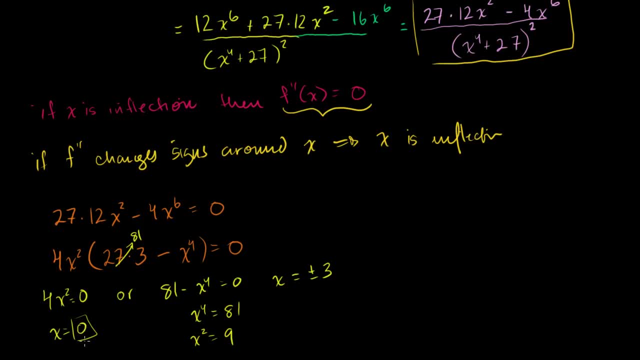 these points in order to be able to label them inflection points. So what happens when x is slightly below 0?? So let's take the situation, let's do all the scenarios. What happens when x is slightly below 0?? Not all of them, necessarily, but if like x is like 0.1, what is the second derivative? 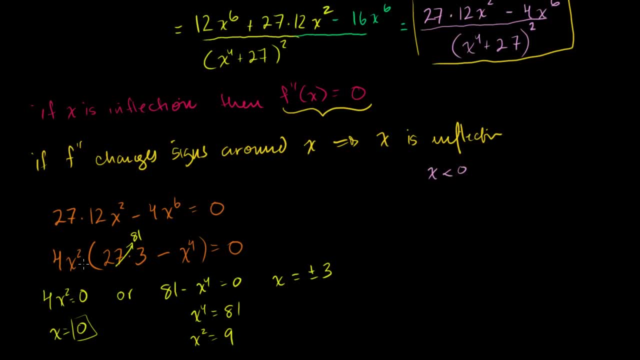 going to be doing. If x is 0.1. This, or if x is minus 0.1, this term right here is going to be positive, And then this is going to be 81 minus 0.1 to the fourth. so that's going to be a very 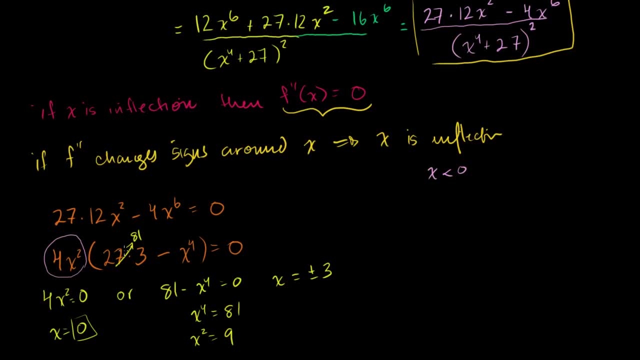 small number, Right. so it's going to be some positive number times 81 minus a small number, So it's going to be a positive number. So when x than 0, or just slightly less than 0,, our second derivative is positive. 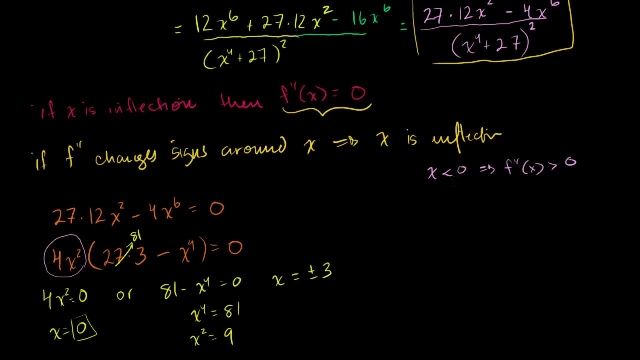 Now what happens when x is slightly larger? When I write this notation, I want to be careful. I mean really just right below 0.. Now, when x is right above 0, what happens? Let's say x was 0.01, or 0.1, positive 0.1.. 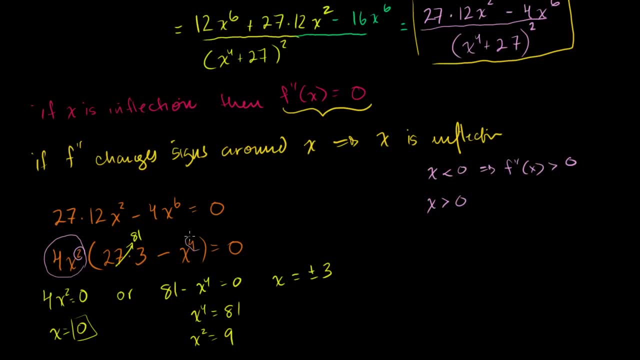 Well, it's going to be the same thing because in both cases we're squaring and we're taking the fourth, so you're kind of losing your sign information. So if x is 0.1, this thing is going to be a small positive. 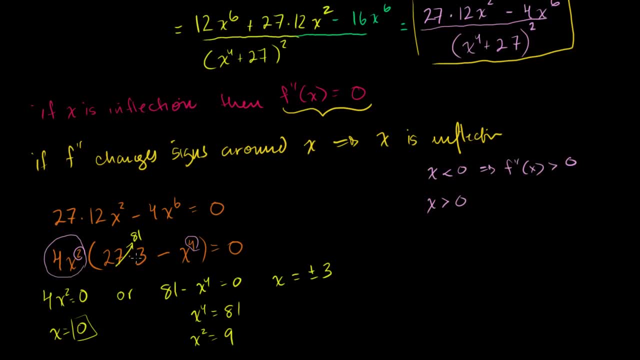 number. you're going to be subtracting a very small positive number from 81, but 81 minus a small number is still going to be positive. So you're going to have a positive times a positive. so your second derivative is still going to. 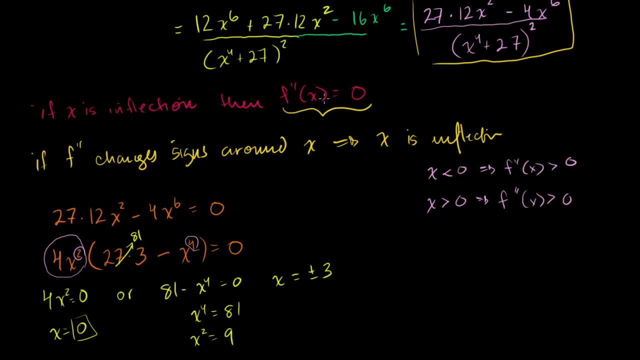 be greater than 0.. So something interesting here: Your second derivative is 0 when x is equal to 0, but it is 0.. It is not an inflection point Because- notice, the concavity did not change around 0.. 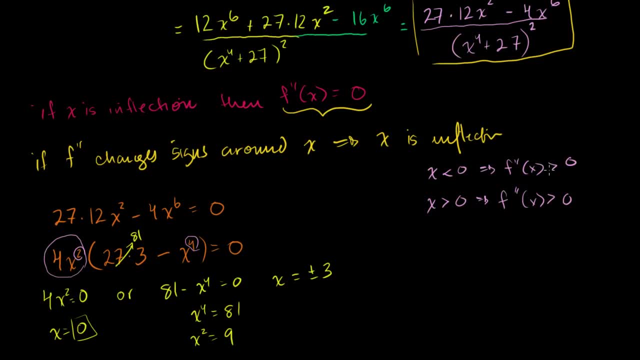 Our second derivative is positive as we approach 0 from the left and it's positive as we approach 0 from the right. So in general at 0, as we're near 0 from either direction, we're going to be concave upwards. 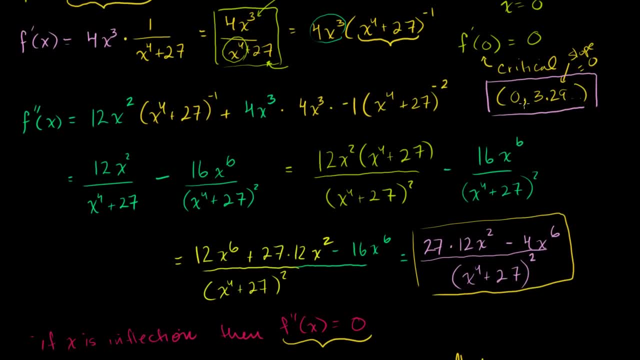 So the fact that 0 is a critical point and that we're always concave upward as we approach 0 from either side, this tells us that this is a minimum point, Because we're concave upwards all around 0. So 0 is not an inflection point. 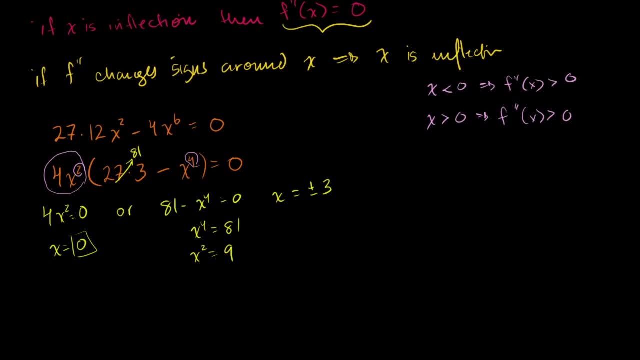 Let's see if positive and negative 3 are inflection points, And if you study this equation, let me write our- and actually I just want to be clear. I've just been using the numerator of the second derivative. The whole second derivative is negative. 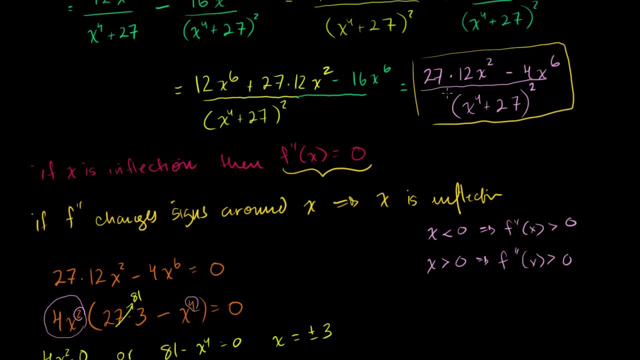 The whole second derivative is this thing right here. But I've been ignoring the denominator, because the denominator is always positive. So if we're trying to understand whether things are positive or negative, we just really have to determine whether the numerator is positive or negative. 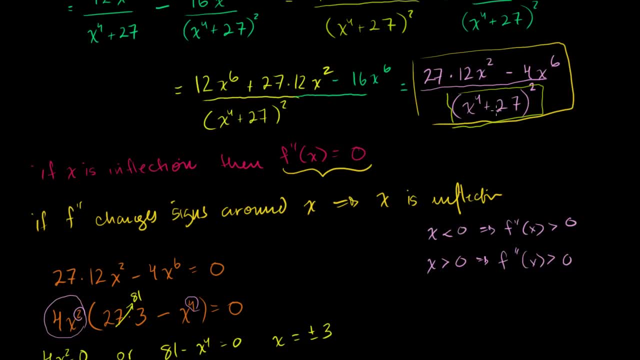 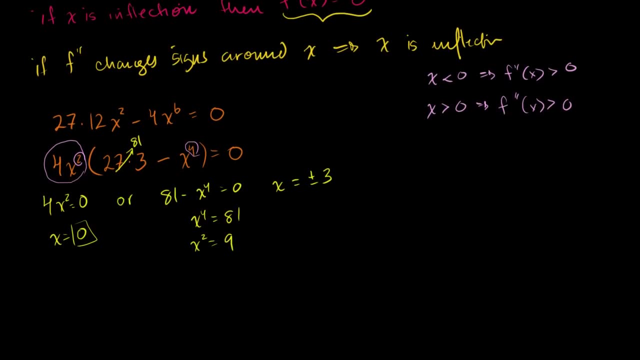 Because this expression right here is always positive. It's something to the second power. So let's test whether we have a change in concavity around. x is equal to positive or negative 3.. So remember the numerator of our. let me just rewrite our. 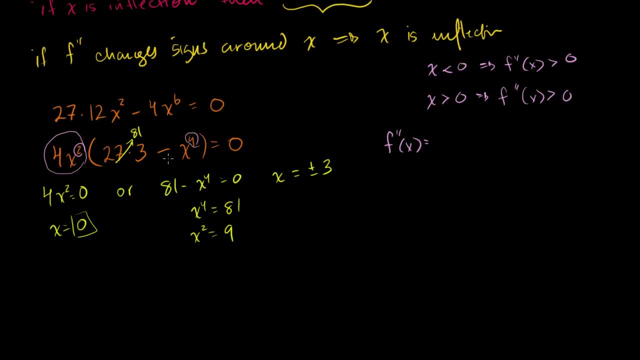 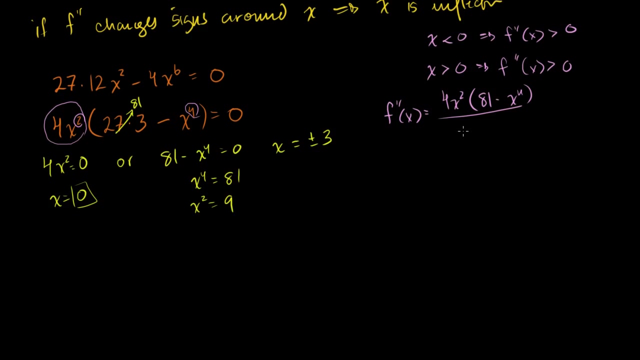 second derivative, just so you see it here: f prime, prime of x. The numerator is this thing: right here It's 4x squared times 81 minus x to the fourth, And the denominator was up here: x to the fourth plus 27 squared. 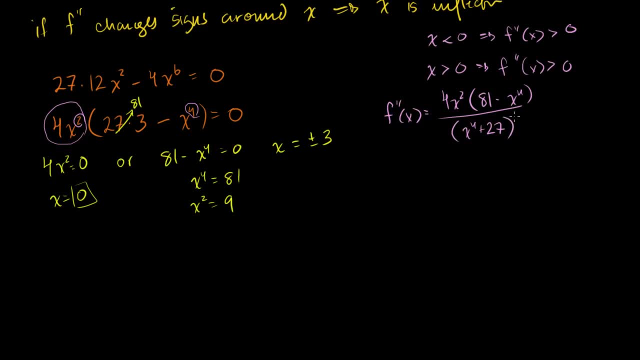 x to the fourth plus 27 squared. That was our second derivative. Let's see if this changes signs around positive or negative 3.. And actually we should get the same answer, because regardless of whether we put positive or negative 3 here, you lose all your sign. 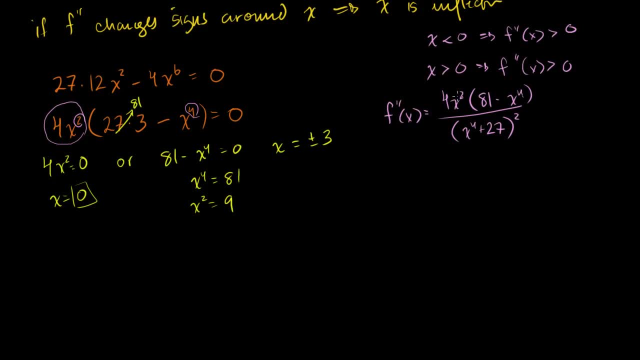 information because you're taking it to the fourth power, You're taking it to the second power And obviously anything to the fourth power is always going to be positive. Anything to the second power is always going to be negative. So when we do our test, if it's true for positive 3, it's 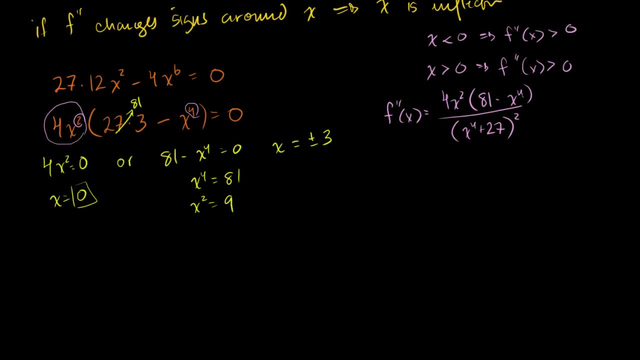 probably going to be true for negative 3 as well, But let's just try it out. So, when x is just a little bit less than positive 3, what's the sine of f, prime prime of x? So it's going to be 4 times 9, or it's going to be 4 times a. 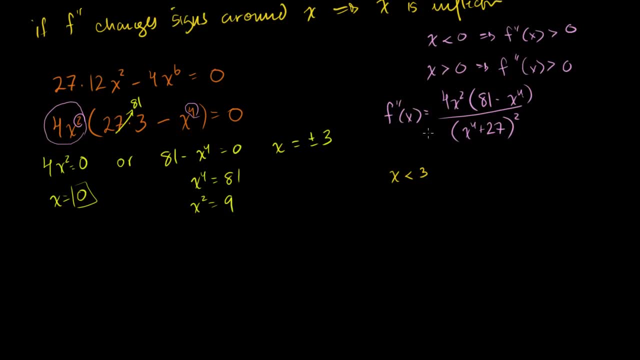 positive number. It might be like 2.999.. But this is still going to be positive. So this is going to be positive when x is approaching 3. And then this is going to be well. if x is 3, this is 0.. 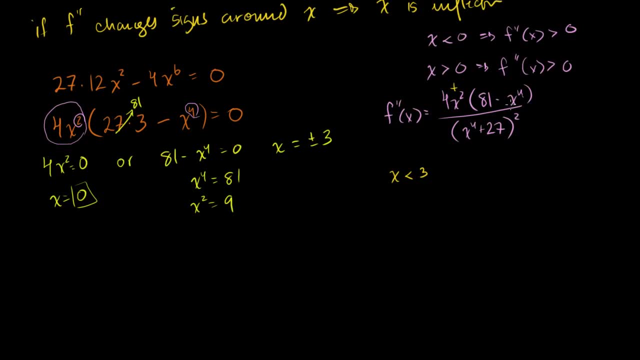 So if x is a little bit less than 3,, if it's like 2.9999,, this number is going to be less than 81. So this is also going to be positive And, of course, the denominator is always positive. 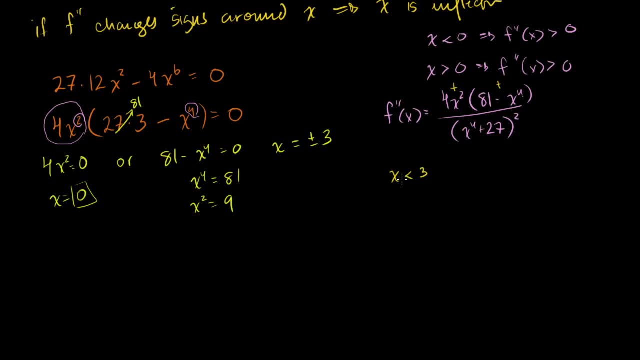 So, as x is less than 3,, as it's approaching from the left, we are concave upwards, This thing's going to be a positive. Then f, prime prime, is greater than 0. We are upwards, concave upwards. When x is just larger than 3, what's going to happen? 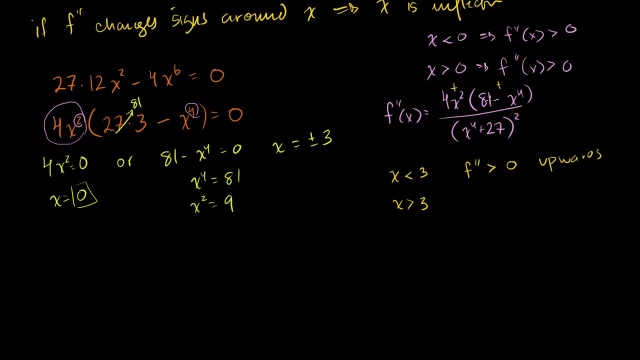 Well, this first term is still going to be positive. But if x is just larger than 3, x to the fourth is going to be just larger than 81. And so this second term is going to be negative in that situation. It's going to be negative when x is larger than 3.. 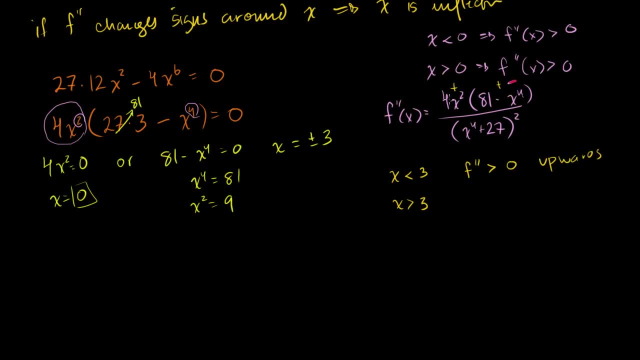 Because this is going to be larger than 81.. So if this is negative and this is positive, then the whole thing is going to be negative, Because this denominator is still going to be positive. So then f prime prime is going to be less than 0.. 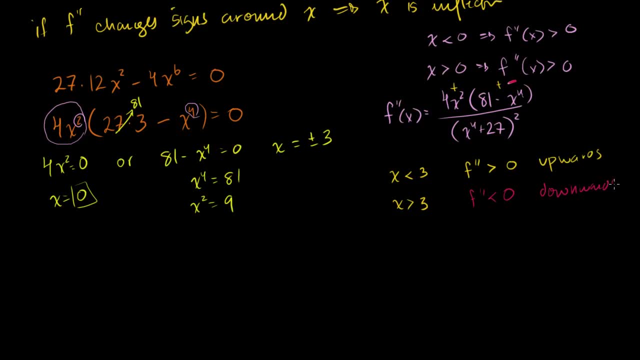 So we're going to be concave downwards. One last one: What happens when x is just greater than minus 3? So just being greater than minus 3, that's like minus 2.99999.. So when you take minus 2.99 and square it, you're going to get. 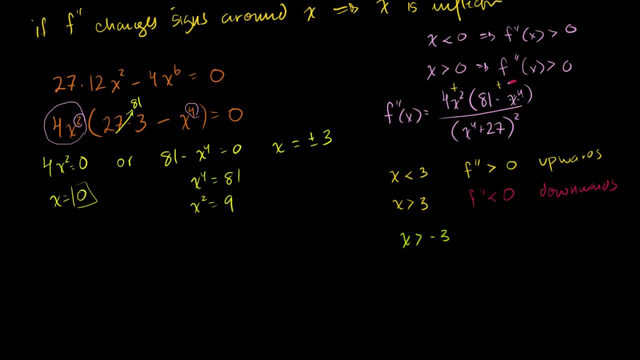 a positive number. So this is going to be positive And if you take minus 2.99 to the fourth, that's going to be a little bit less than 81.. Because 2.99 to the fourth is a little bit less than 81.. 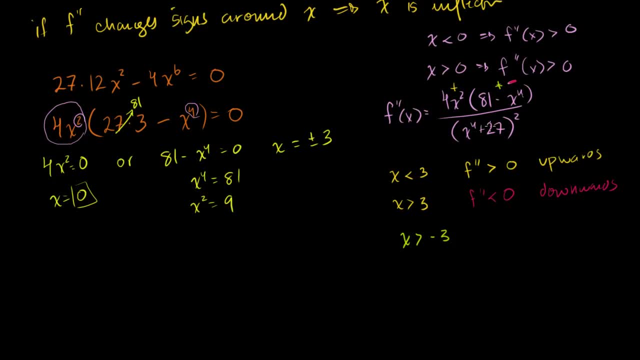 So this is still going to be positive. So you have positive times, a positive divided by a positive. So you're going to be concave upwards Because your second derivative is going to be greater than 0.. Concave upwards And then, finally, when x is just less than negative, 3.. 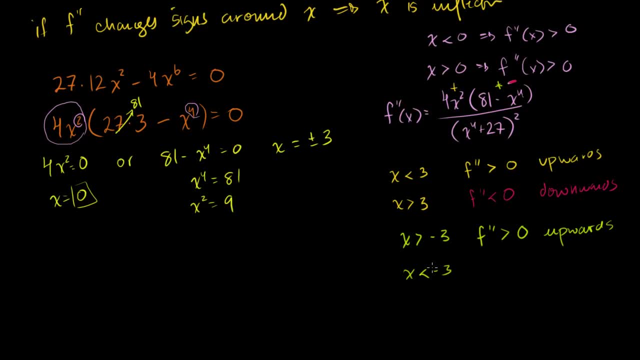 Remember, when I write this, I don't mean for all x's larger than negative 3 or all x's smaller than negative 3.. I'm really. there's actually no well, I can't think of the notation that would say, just as we just approached 3, in. 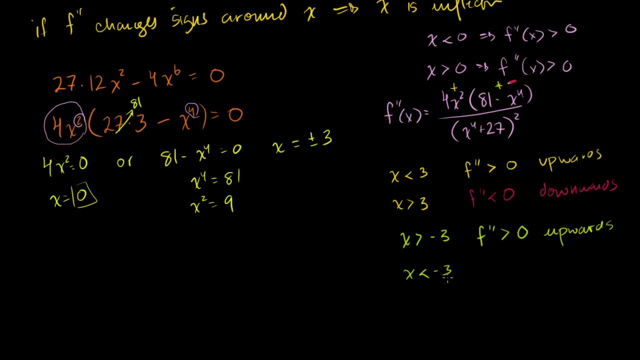 this case from the left. But what happens if we just go to minus 3.11? Or 3.01,, I guess is a better one- Or 3.1.. Well, this term right here is going to be positive. 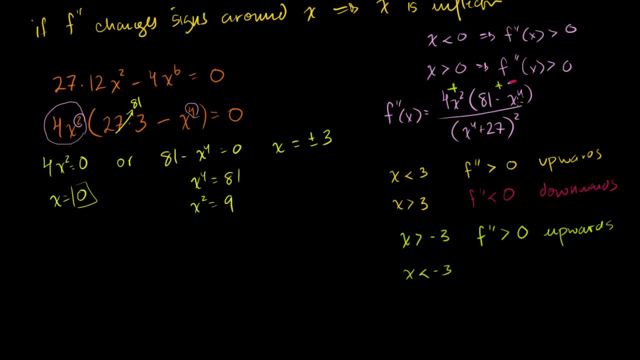 But if we take minus 3.1 to the third, that's going to be larger than positive 81,. right, The sign will become positive. It'll be larger than 81. So this will become negative. So in that case as well, we'll have a positive times a. 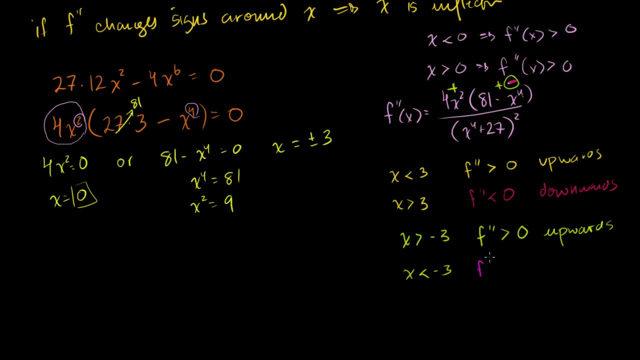 negative divided by a positive. So then our second derivative is going to be negative, And so we're going to be downwards. So I think we're ready to plot. So, first of all, is x plus or minus 3 inflection points? 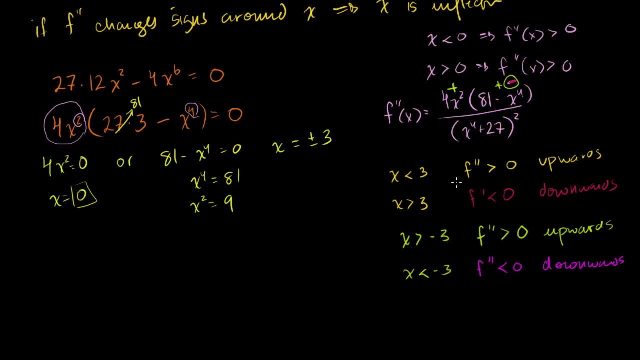 Sure, As we approach, x is equal to 3. from the left, We are concave upwards, And then, as we cross 3, the second derivative is 0. I lost it up here. The second derivative is 0. And then, as we go to the right, of 3, we 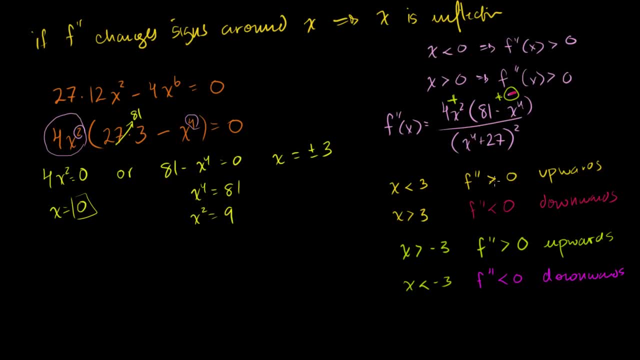 become concave downwards. So we got our sign change in the second derivative. So x is equal to 3.. So this 3 is definitely an inflection point, And the same argument could be made for negative 3.. We switch signs as we cross 3.. 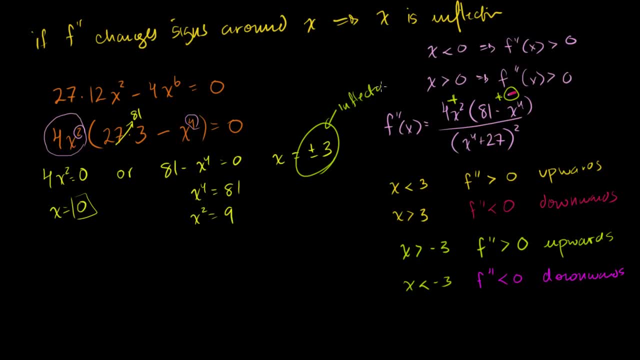 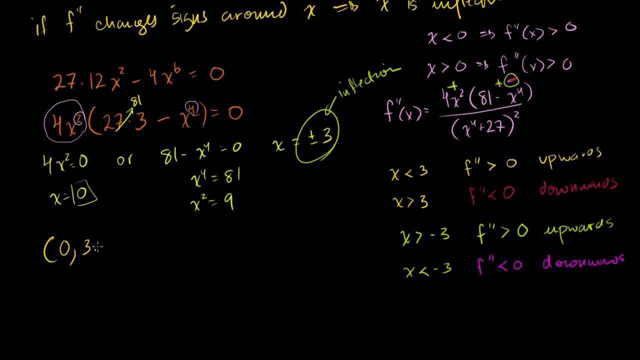 So these definitely are inflection points. And just so we get the exact coordinates, let's figure out what f of 3 is, or f of positive and negative 3.. And then we're ready to graph. So first of all, we know that the point 0, 3.29,, that this 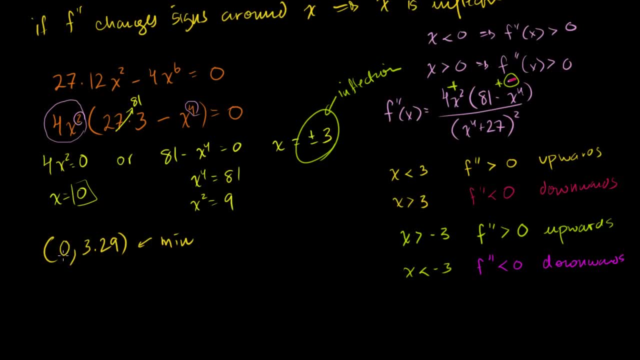 was a minimum Because 0 was a critical point. the slope is 0 there And because it's concave upwards all around 0. So 0 is definitely not an inflection point. And then we know that the points positive 3 and minus. 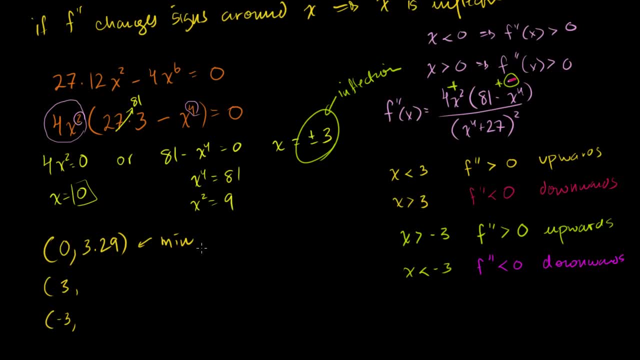 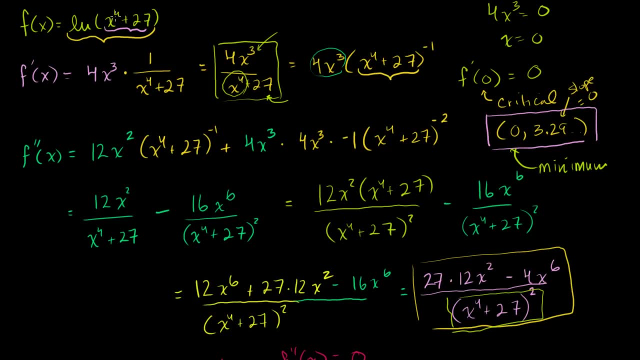 3 are inflection points And in order to figure out their y-coordinates, we can just evaluate them. So they're actually going to have the same y-coordinates, Because if you put a minus 3 or a positive 3 and take it to, 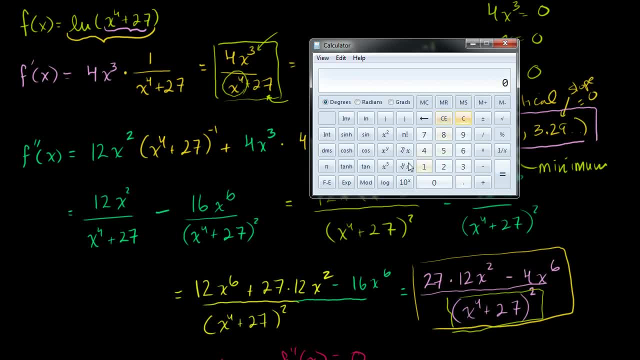 the fourth power, you're going to get the same thing. Let's figure out what they are. So if we take 3 to the fourth power, that's what 81.. 81 plus 27 is equal to 108.. And then we want to take the natural log of it. 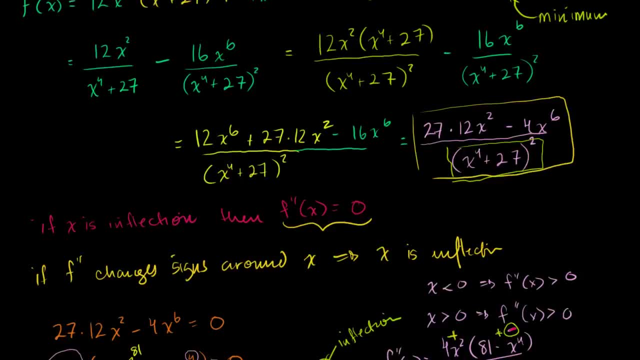 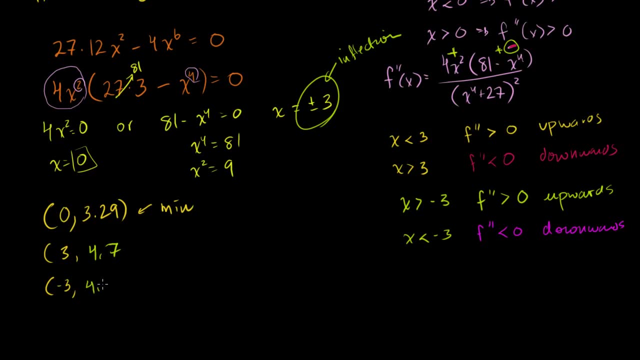 Let's just say 4.7.. Just to get around, It's a rough idea- 4.7.. And that's true of whether we do positive or negative 3, because we took it to the fourth power, So it's 4.7.. 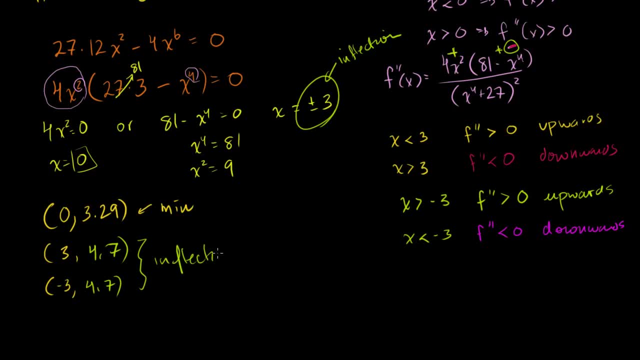 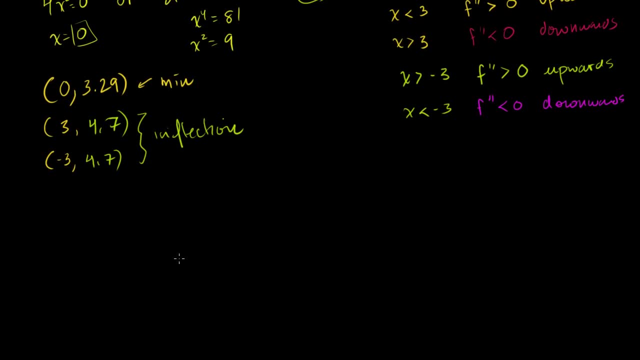 These are both inflection points And we should be ready to graph it. Let's graph it. All right, Let me draw my axis. Let me draw my axis, just like that, And then this is my y-axis, This is my x-axis. 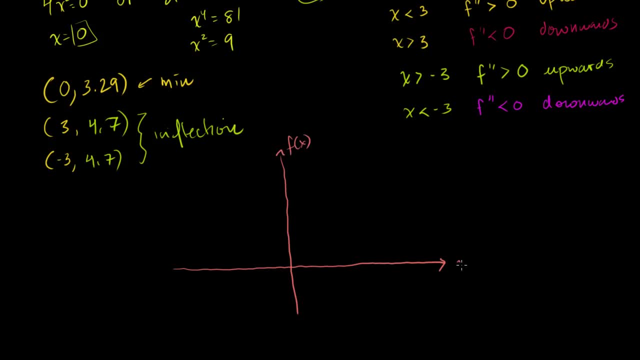 This is y. You could even call it the f of x-axis, if you like. This is x, And so the point 0, 3.29.. So let's say this is 1, 2, 3,, 4, 5.. 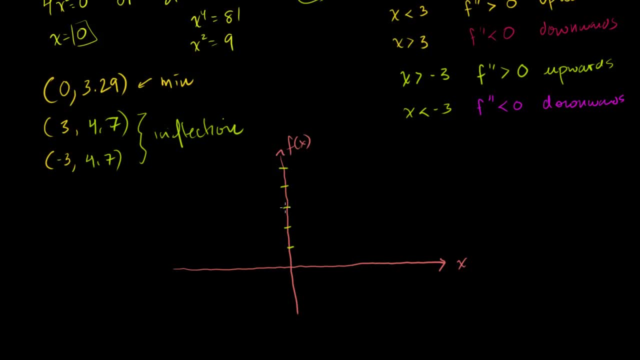 So the point 0, 3.29.. So it's 0, 1,, 2, 3, a little bit above 3 is right there. That's the minimum point And then we're concave. The slope is 0, right there. 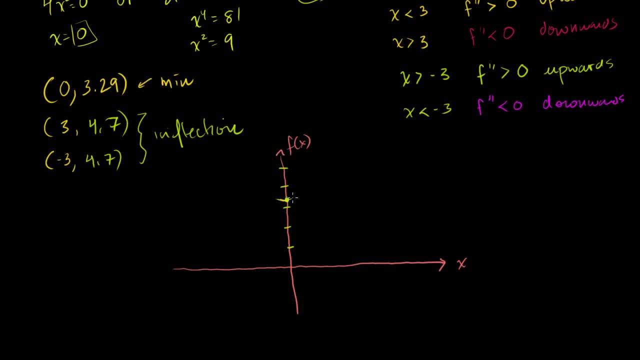 We figured that out because the first derivative was 0 there. so it's a critical point And it's concave upwards around there. So that told us we're at a minimum point right there And then at positive 3.. So 1,, 2,, 3.. 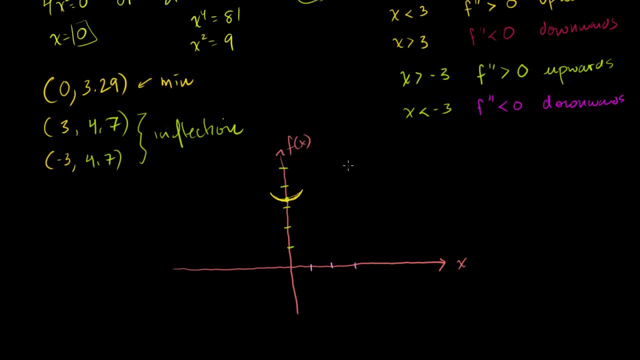 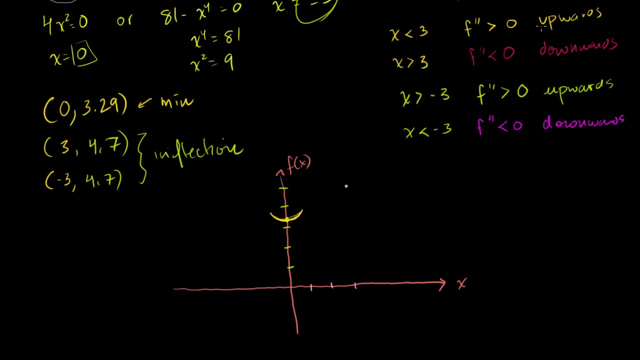 At positive 3, 4.7.. So 4.7 will look something like that: We have an inflection point, Before that we're concave upwards And then after that we're concave downwards. So it looks something like this: 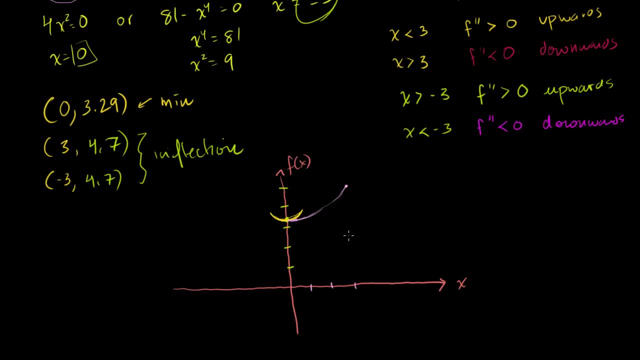 So we're concave upwards up to that point. Maybe actually you should let me ignore that yellow. It's the same thing I drew before. Let me get rid of that. So let me draw it like 1,, 2,, 3.. 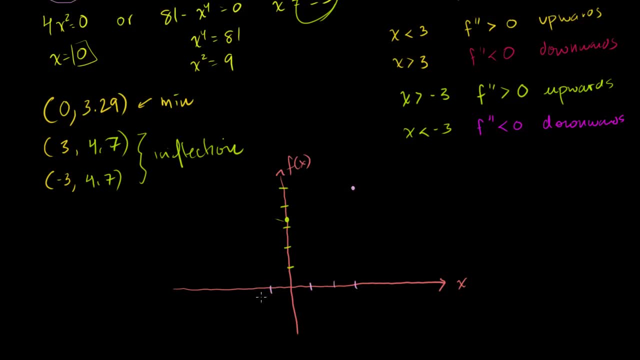 3, 4.7 looks like that, And minus 3, 4.7.. 1, 2, 3.. 4.7 looks like that. So we know, at 0, we have a slope of 0..